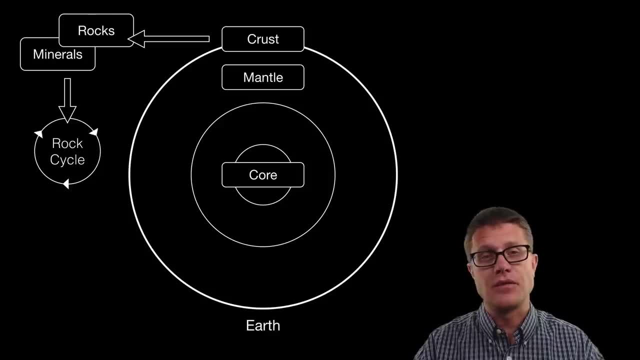 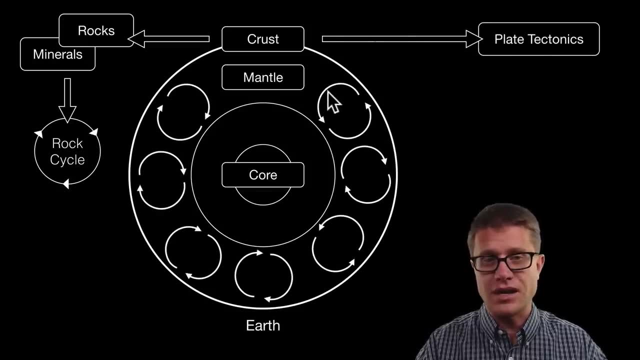 that through the rock cycle. Now the crust itself is made up of these large continental and oceanic plates And they float on the mantle itself, And so this is rock under here, but it is rock that is moving As we generate heat. as it moves up, it is pushing those. 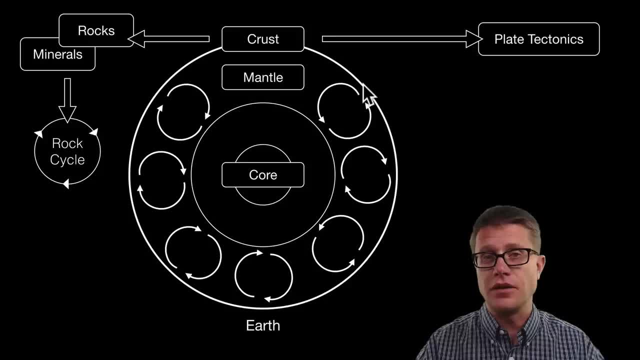 plates around. They move very slowly, about the same rate that your fingernails grow before huge impacts, And so when those plates run into each other, we have boundaries. An example of that would be the ring of fire. So if you look around the Pacific Ocean, you 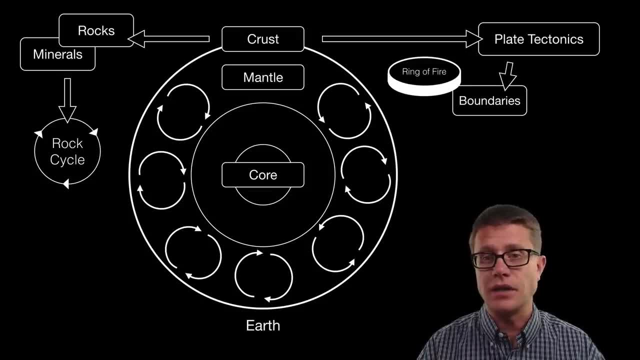 have this area where almost all the earthquakes and volcanoes take place. We also have what are called hot spots, And those are going to be areas where a plate will move over a hot area in the mantle and we can form islands like Hawaii. Now, if we look at where those 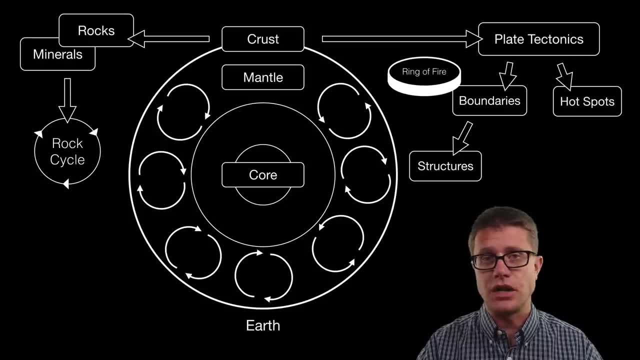 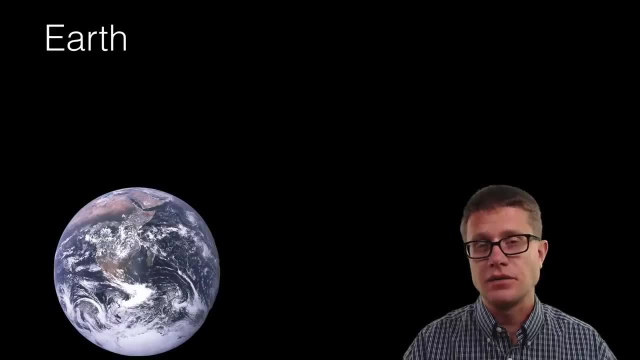 boundaries occur, we will have structures like volcanoes and mountain chains, But we also, therefore, have hazards around those areas Where it can impact the earth And we know it can impact human society, and we will discuss a lot of those. And so to understand what, 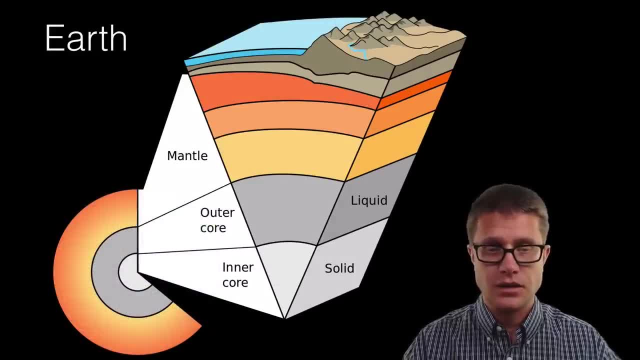 is going on in the earth, we should really understand what it looks like on the inside. So we have a solid inner core, a liquid outer core, and then we have what is called the mantle. Now, around 85% of the volume of the earth is going to be in this mantle, And so it is. 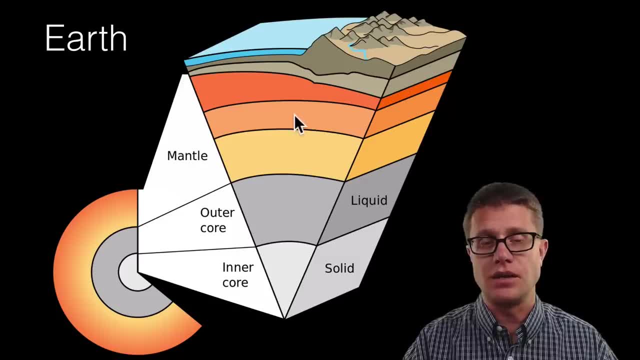 rock, but it is rock that is moving. We are generating a huge amount of heat down here, And then we finally get up to what is called the crust. That is where we live, And so on that crust we have rocks, And those rocks are: 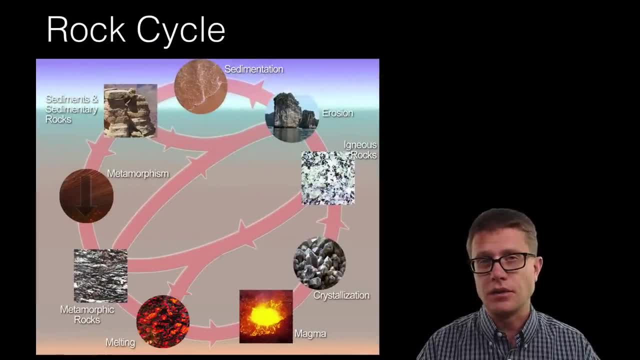 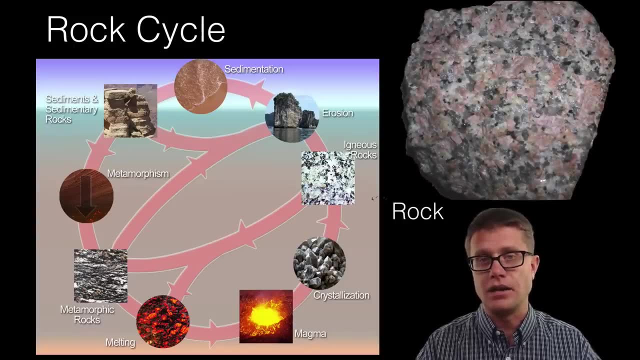 constantly being shaped from one end to another, And so if we take a look at this rock cycle- since it is a cycle you could start anywhere- Let's start with an igneous rock. So an igneous rock, like granite, is going to be formed when we have crystallization of magma. So, as it 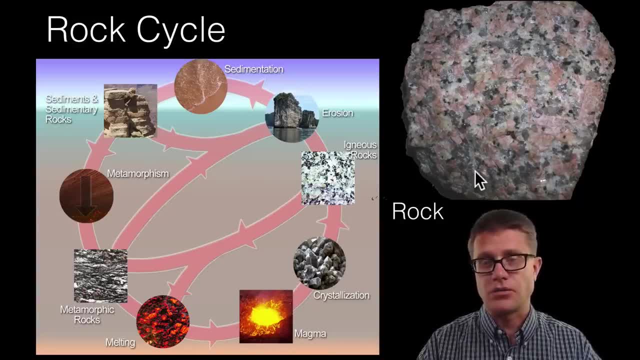 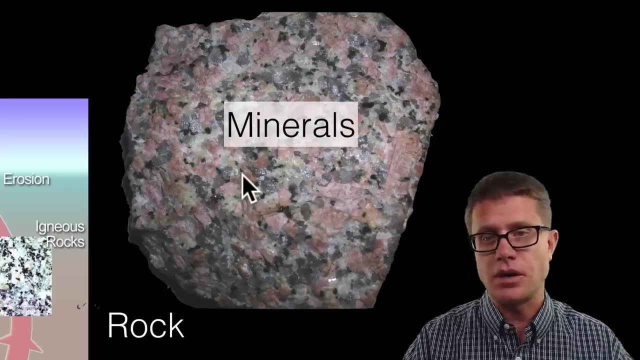 crystallizes. you can see those crystals right here. So this granite is made up of minerals. So I can see, for example, this quartz and this pink feldspar And we have this mica. So these are the minerals that make up the rock itself. 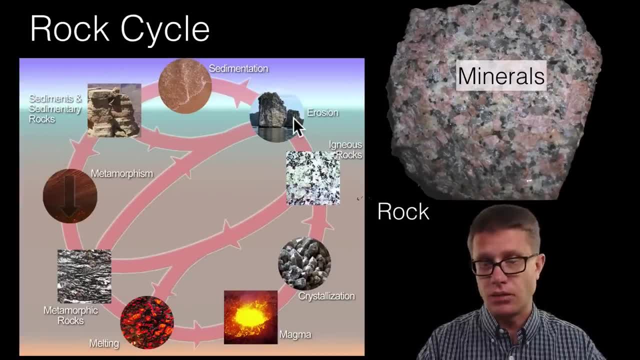 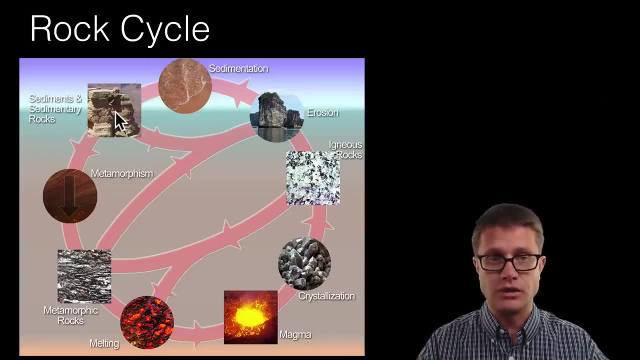 But this could experience erosion. So erosion on the planet- water, wind- can cause it to break down into sediments And therefore, after it has done that, it could get squeezed for a long period of time and we could have a sedimentary rock which is going to be compressed. 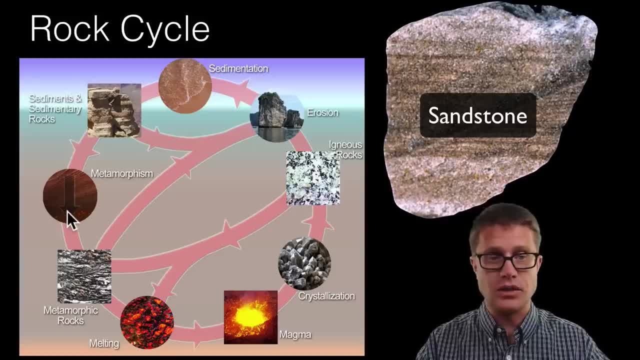 sediments. Now that could be squeezed. We could squeeze it under the surface of the earth using heat and pressure. It could form something like quartzite. Or we could take that igneous and we could squeeze it and make something like gne, And so gne is gne, And 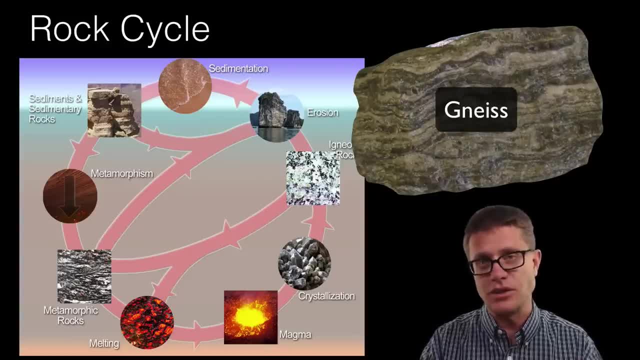 gne is a type of metamorphic rock that is formed by the squeezing of granite. Now you can see those minerals are still there, but it has a different shape, And so the rocks on our planet are continually recycled, over and, over and over again. But if we get back, 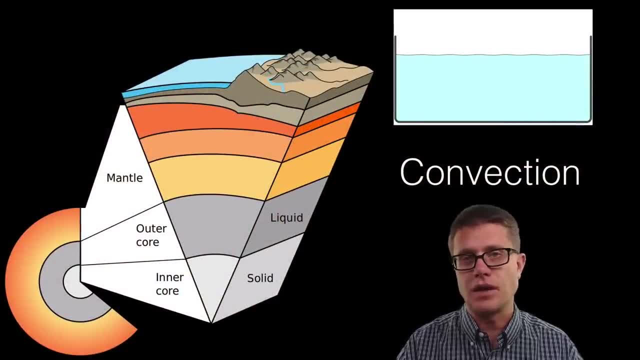 to the structure of the earth. what is driving all of this are going to be convection currents within the mantle itself, And so if you look at this and say, this is some boiling water. So if we generate a little bit of heat underneath it, that heat is going to be transferred through. 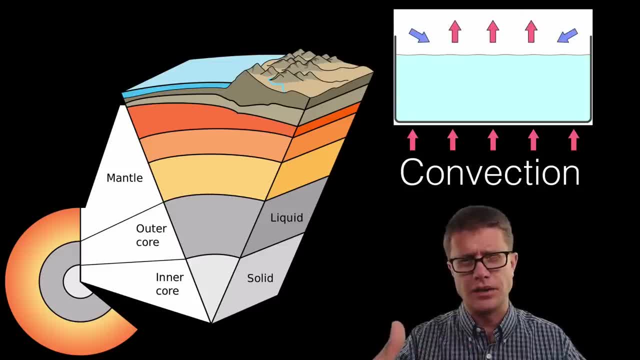 the water. So if you held your hand up here, you would feel some of that heat up there Above it. But if we look inside the water itself, we are going to have these convection currents, Areas where we are heating it up, And so we are decreasing the density, and then 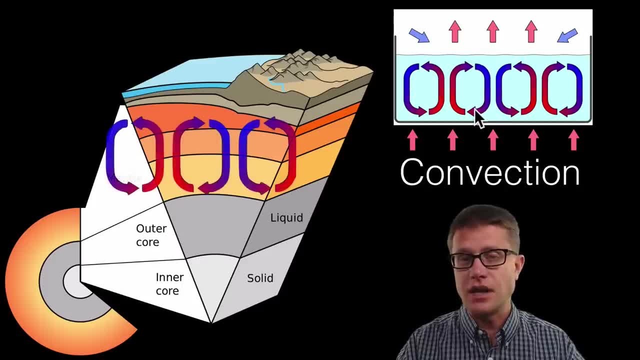 it cools down and then it is going to sink again, And so we are going to find the same thing in the mantle itself. It does not occur as quickly as it does in the boiling water, But it has huge implications on the crust above, And so if we look at that crust, it 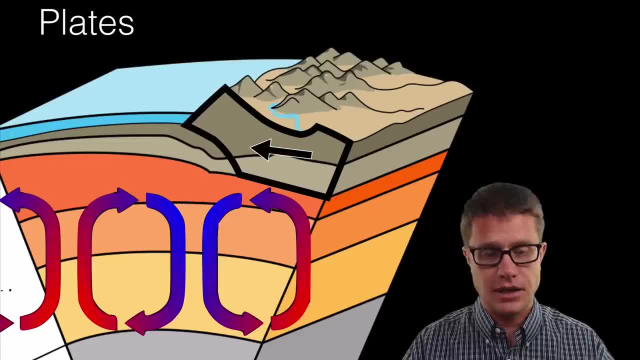 is actually made up of plates, And so if I trace out a plate like this, this would be a continental plate, And so it is being pushed to the left, And the reason why it is being pushed is because of this convection current is moving like that. It. 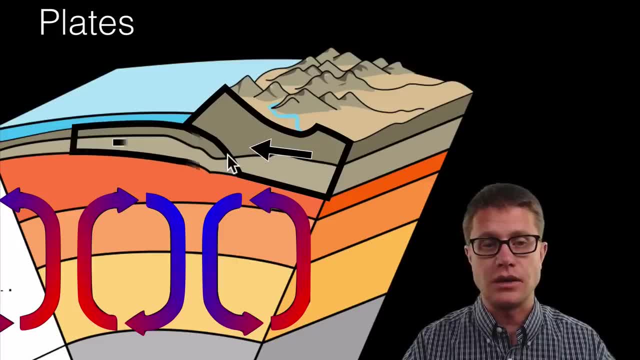 is forcing the plate in that direction And it is running into another plate. So we have an oceanic plate. The oceanic plates are going to be more dense and they will be pushed underneath a continental plate, And what we are going to get right along this margin is going to 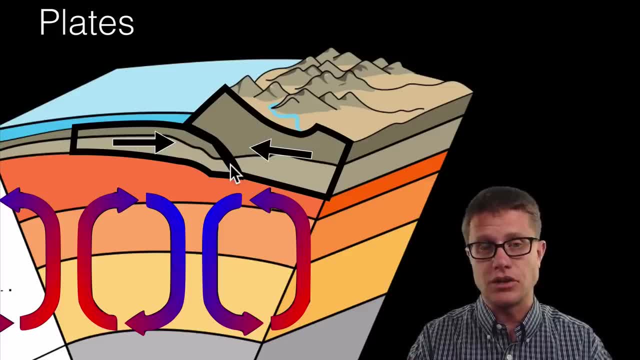 be a convergent plate boundary. They are running into each other, But we could look over here and maybe there is another oceanic plate that is moving in the other direction. Why is it moving in the other direction? Because the convection current is pushing it here And 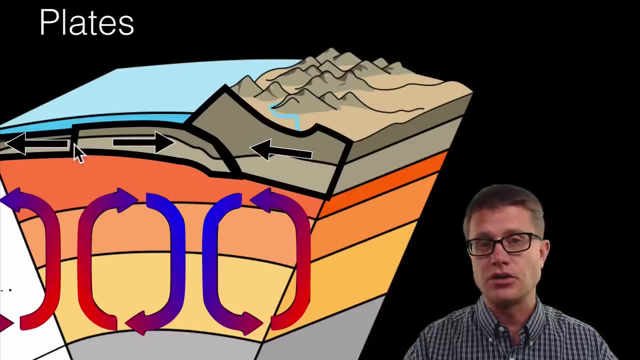 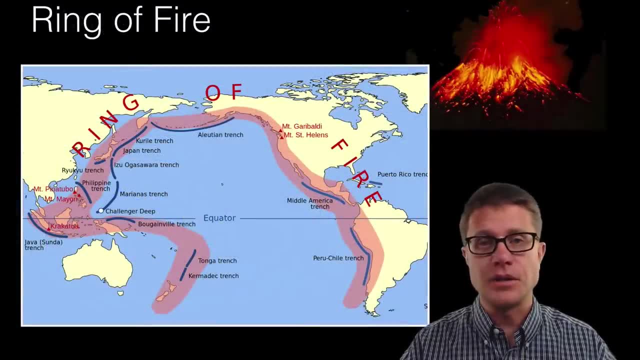 pushing it there, And so we could have this mid-Atlantic ridge or this mid-oceanic ridge being formed right there. So we have known this for a long time. If you look at the ring of fire we find around the Pacific Ocean, we have an aggregation of volcanoes and earthquakes. 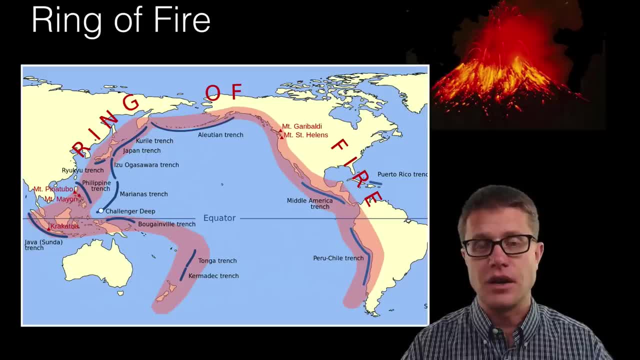 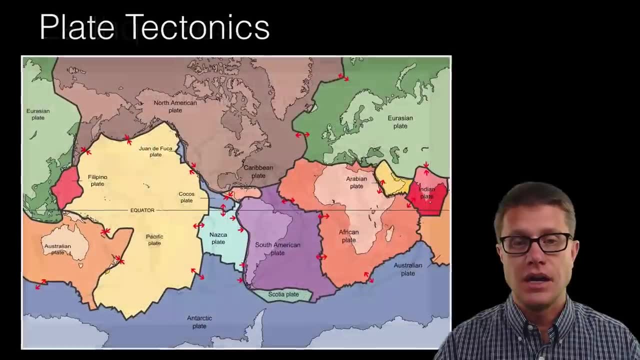 Something like 75% of all volcanoes, 90% of earthquakes, are found in this area. If we start plotting where those earthquakes are, we can start to see where those plates exist. And if we look at the plates on our planet, it is hard to wrap your head around this picture. for a second. So this is North America right here, And if we look at the plates on our planet, it is hard to wrap your head around this picture for a second. So this is North America right here, And if we look at the plates on our planet, it is hard to wrap your head around this picture for a second. So this is North America right here, And 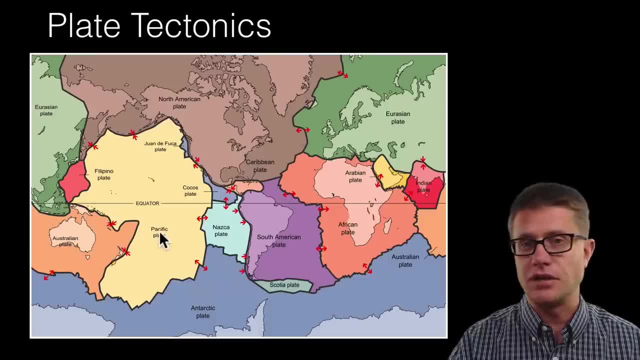 if we look at the plates on our planet, it is hard to wrap your head around this picture for a second. So this is North America right here, And then it sits on this giant North American plate, And then we would have the Pacific plate. 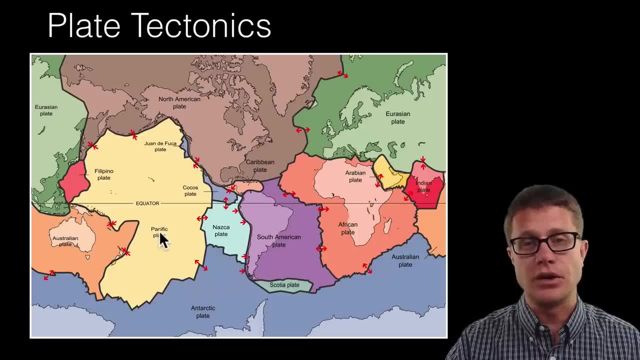 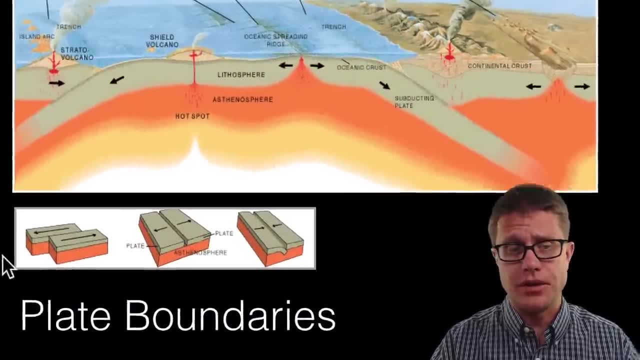 right here, And so those plates are constantly moving around. You are probably familiar with Pangea, which was a time when all the continental plates had come together. So what happens when plates meet is that they can do one of three things. They can slide past one another. 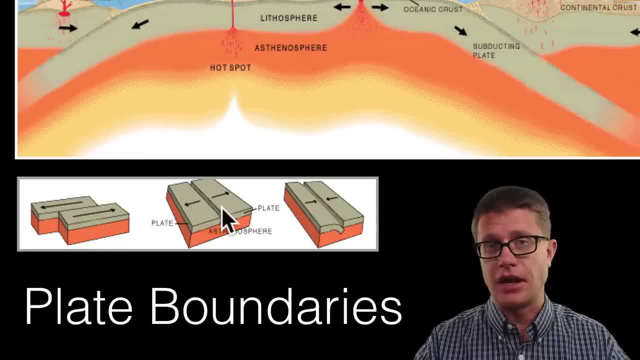 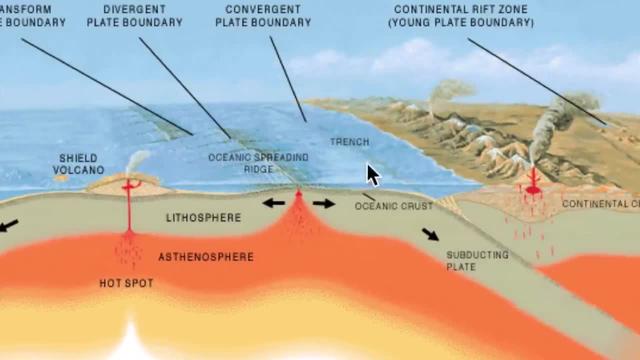 in this transform boundary. They can move apart- We call that a diverging boundary- Or they can run into each other. That is converging. And so if we look at an example of that, right here we have a convergent plate boundary. So what is going on? We have got this oceanic 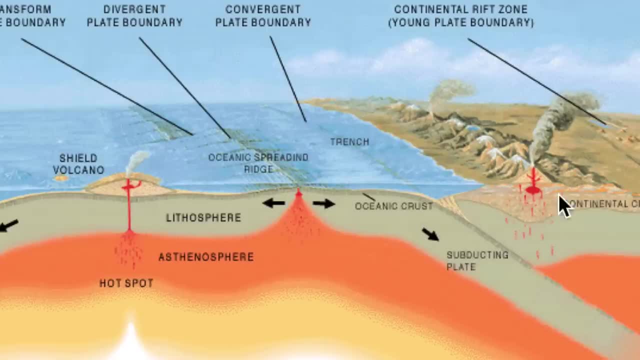 plate, which is being pushed or subducted underneath the continental plate. I described that just a second ago. What is happening is we are melting that rock and that is forming this volcano chain that goes all the way back here. An example could be the Cascades in Washington. 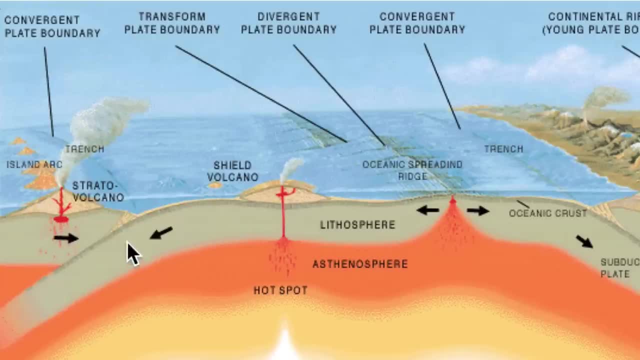 State. We could also have a convergent boundary right here where we have an oceanic plate going underneath another oceanic plate And we get this island arc. like the Aleutian Islands in Alaska. We could have divergent boundaries. An example could be right here. So we have this oceanic 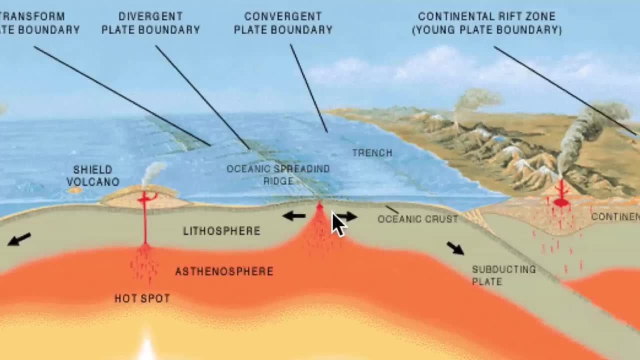 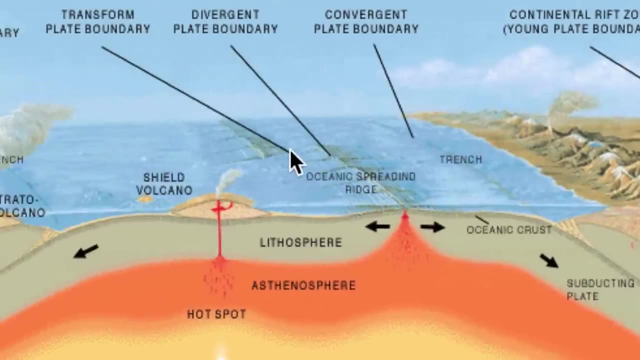 plate, moving away from this oceanic plate So we get this mid-oceanic ridge. We could have a rift valley where this continental plate is being pulled apart. We could have transform boundaries. Here would be an example where they are sliding past one another, San. 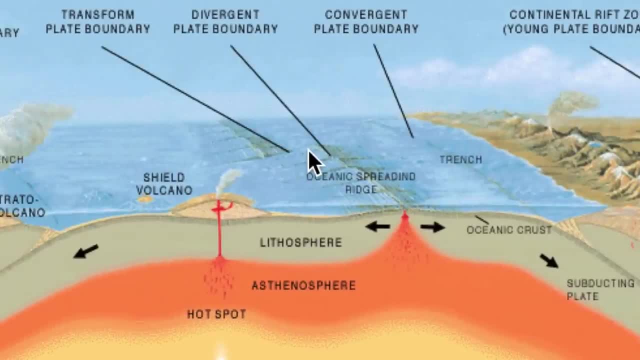 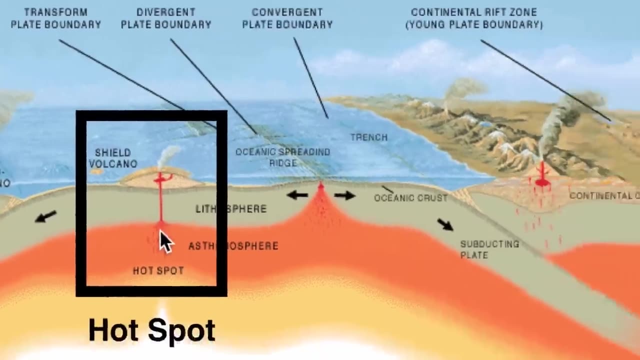 Andreas Fault is a good example of that, But we could also have structures where there is no boundary. So, if we look right here, we have what is called a hot spot. Remember, that is going to be an area where the mantle is close to the surface, And so, for example, Hawaii. 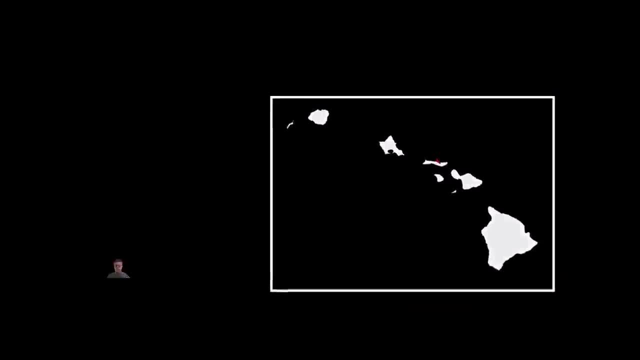 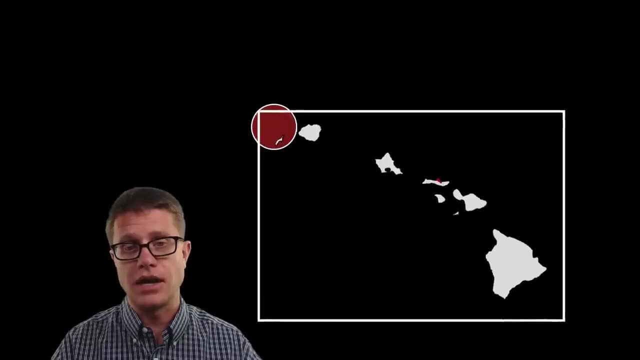 was formed As the plate slid over a hot spot, And let me show you what that looks like. So if we imagine that is the hot spot, It is going to be underneath the plate. And what has happened to Hawaii over time is it slowly slid over the hot spot. The hot spot stays in the same. 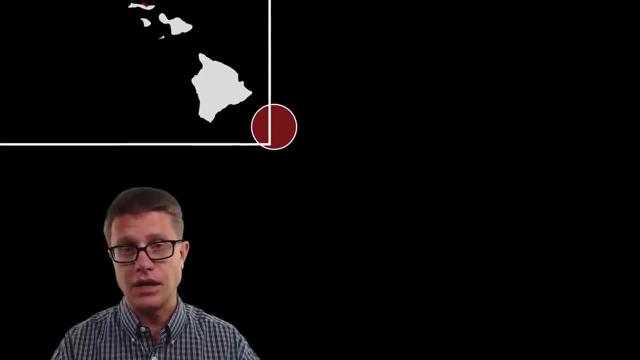 location, And so we have volcano after volcano, after volcano, And so this is the most recent volcano And we will have another island right here, And the reason there are smaller islands out here is that there is more erosion. Yellowstone National Park is another example of a hot spot. 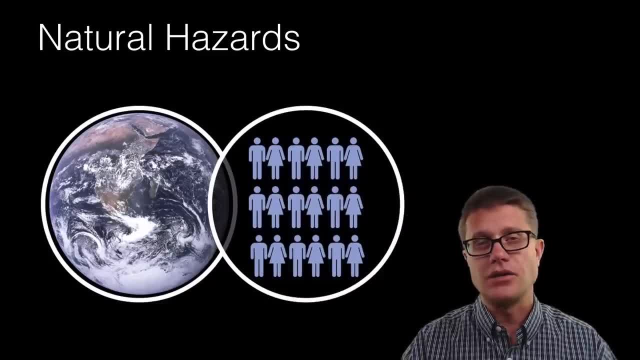 and the plate simply sliding over the surface. Now we get to humans and human society and how we start to interact with the structures of the earth, And so living around these boundaries can be dangerous. It is just a matter of time. So an example could be volcanoes, Some volcanoes. 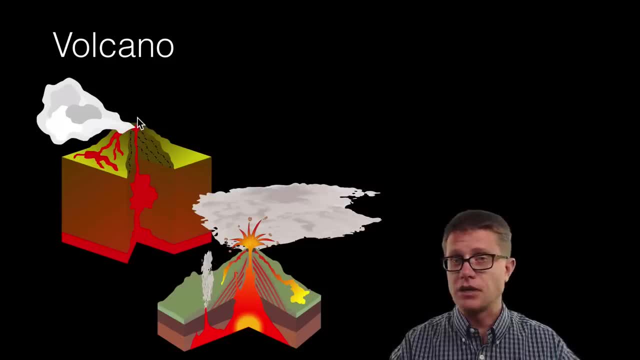 like the ones we would find in Hawaii, can ooze out, And as long as we are able to move out of there quickly, we are going to be fine. But some are highly explosive And it depends on what minerals make up that rock that determines the explosiveness of the volcano- A very explosive. 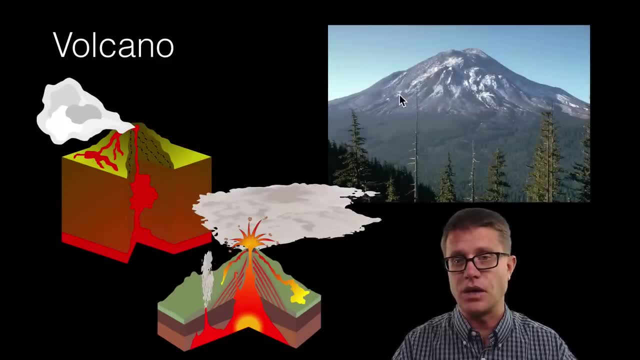 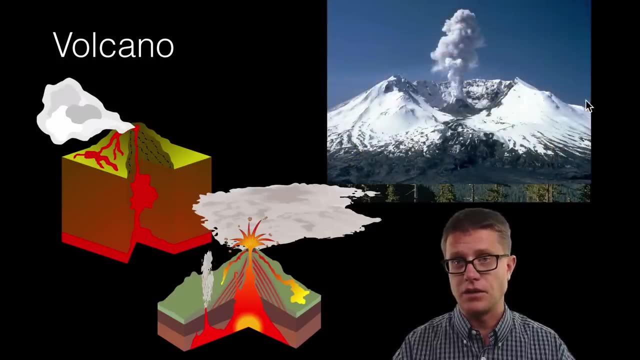 one I remember is Mount Saint Helens, And so this is a picture of Mount Saint Helens in Washington. This is the day before it exploded, And so just take a second to imagine. that is the structure of the volcano, and now it is gone and rebuilding again, And so it literally. 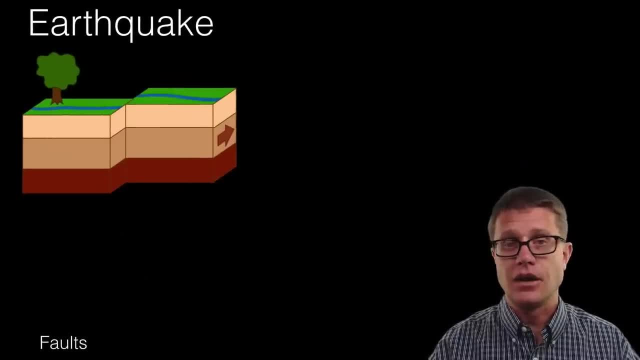 blew apart And if you were on or near that, you died. Earthquakes are another example of a natural hazard. What we have are faults, And this would be a fault right here, And we have one plate, in this case, transform fault where it is sliding past, one We could. 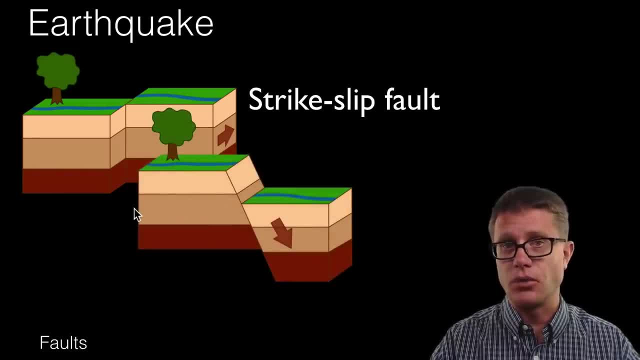 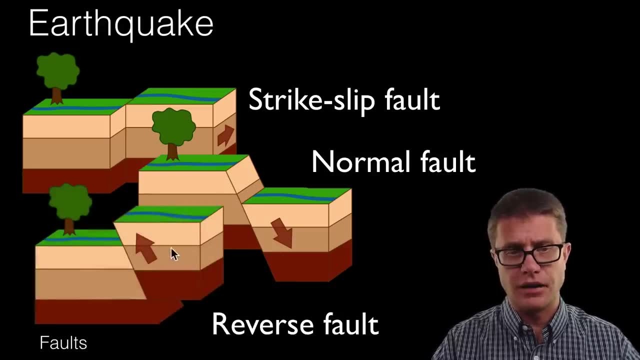 also have a divergent boundary, So these two are moving away from each other, And so we have what is called a normal fault: It is slipping down. Or we could have a reverse or thrust fault when we have a convergent between these two areas on either side of 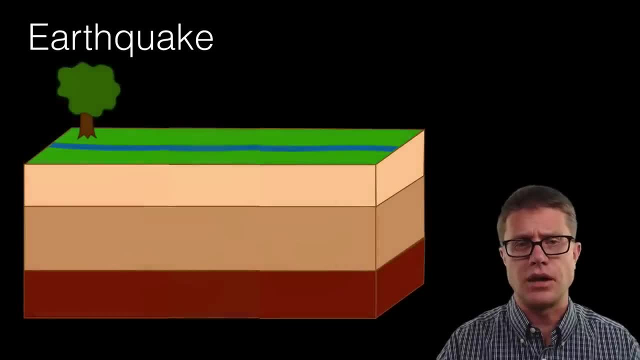 the fault. Now, the names are not as important in really understanding what is going on in an earthquake. If you think about it, if we have two plates that are pushing on each other, eventually they are going to build up pressure and it is going to slip, And as it does, that, 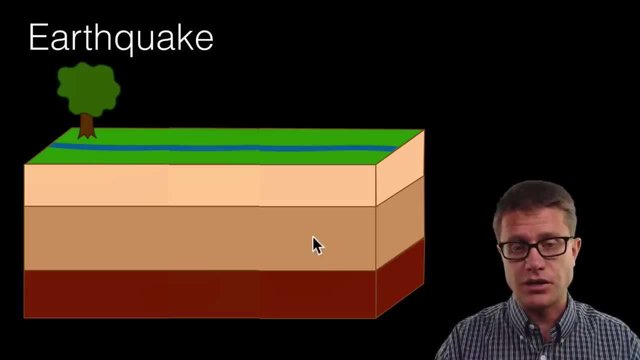 we have an earthquake. So if we watch this right here, let's say there is pressure in this direction and this direction, And then we have a divergent boundary, And then we have a collision And eventually it builds up and we have a slide along that fault line. 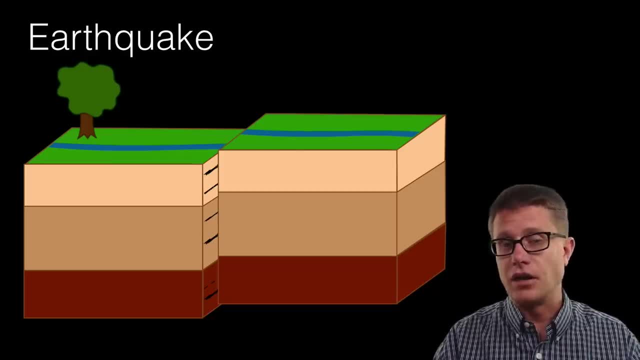 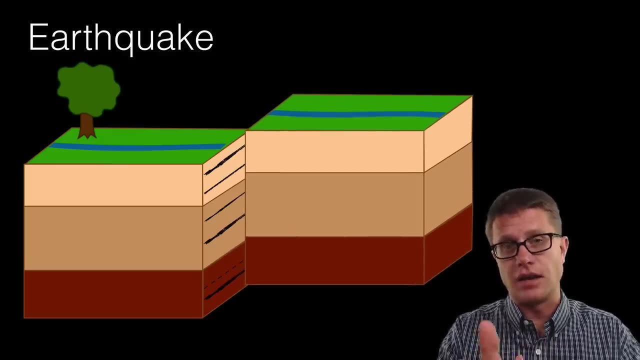 Now it is not like it stopped. There is still pressure there. We could have another earthquake in the future And another earthquake in the future As these move past each other. it is just going to move in small slips And every time we do, we have an earthquake. Now, if you 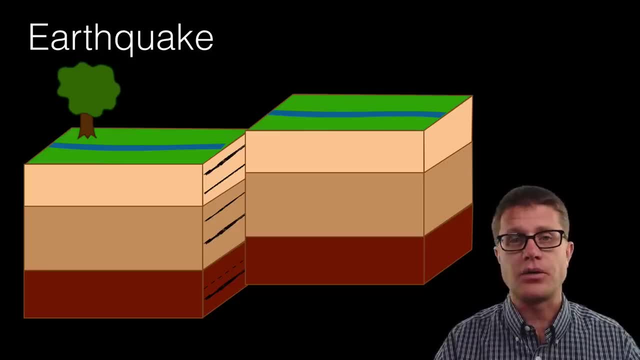 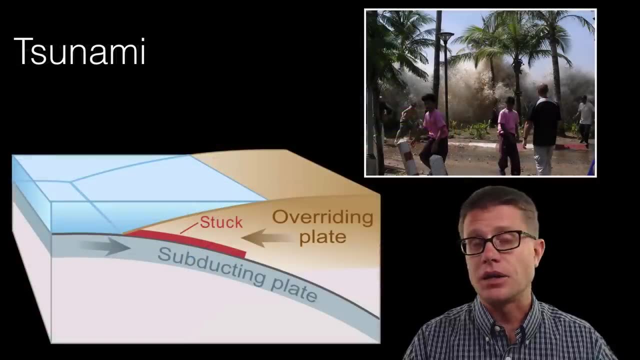 are standing on the surface and there is an earthquake, you are going to be fine. The problem is, if we build structures on that and it is not earthquake ready, then those fall in and humans are going to be impacted. We could also look at tsunamis which are caused by 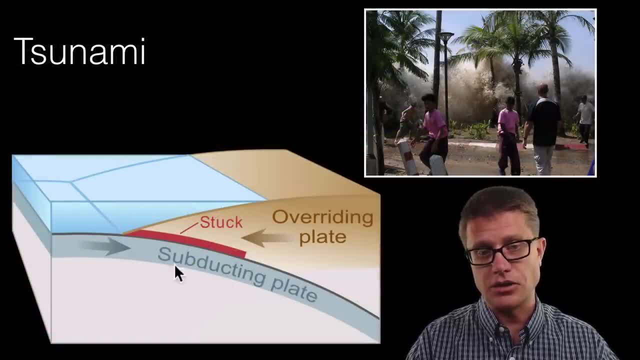 earthquakes. We could also look at earthquakes which are caused by earthquakes. We could also look at earthquakes which are caused by earthquakes. We could also look at earthquakes. What we have got here is a subducting oceanic plate. This would be a continental plate. 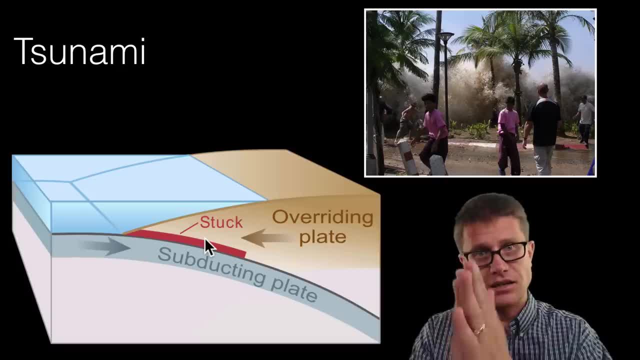 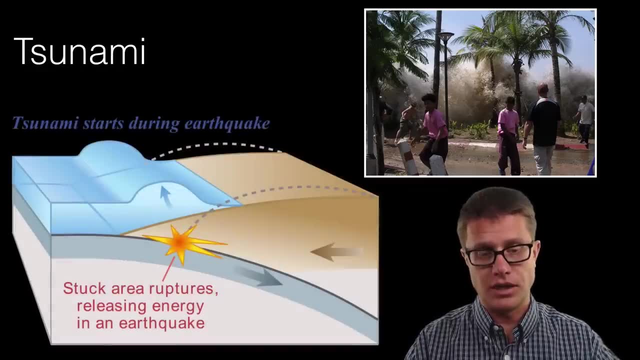 And what is happening is this is being pushed underneath, but it will just stick, And so it is not going to release. And as it sticks, then we build up pressure And then eventually, when it slips, what we get is a huge push up on the water above it. So you get this vertical. 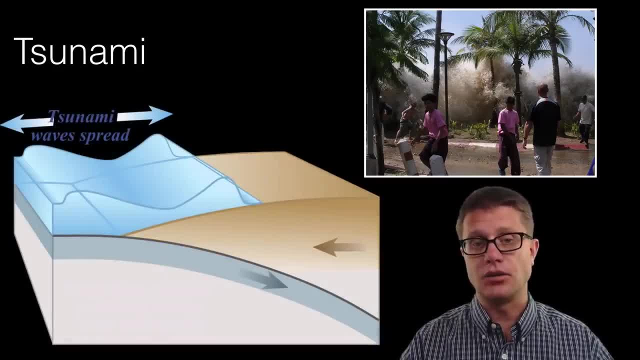 motion in the ocean And that leads to these giant tidal waves. And so if you are near the ocean, you would also suddenly notice that the ocean is going way out, And then you would notice there is a big wave of water coming in And then it is going to come way in And 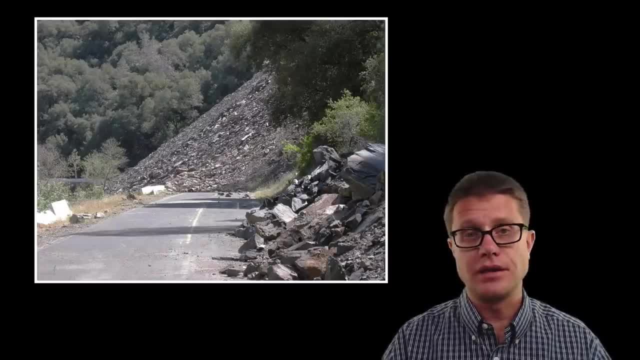 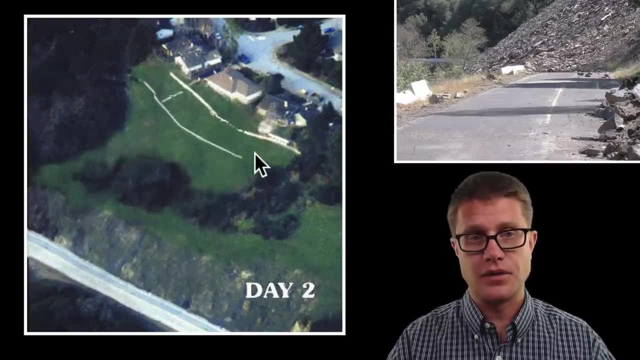 there are really bad consequences from that. We could also have mass wasting. So an example could be a landslide moving across this road. This is a picture taken before and then watch it after. a landslide- Now it does not occur really quickly. It could be triggered by an. 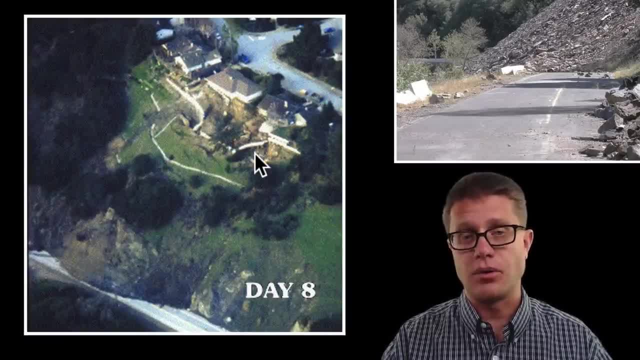 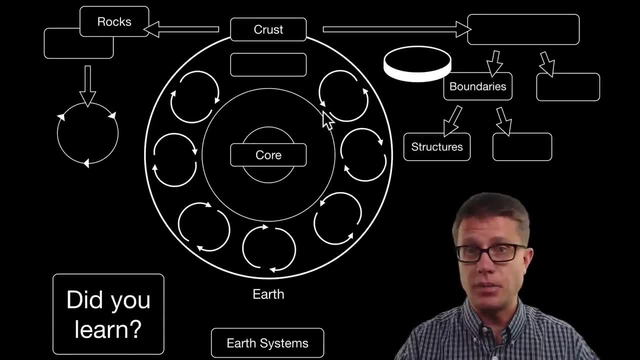 earthquake, But generally, if we get a lot of water in an area, it cannot support that wave, And so did you learn about earth systems, Do you? can you stop the video and try to fill in the blanks? right now I would pause the video, But if not, I would take a break. 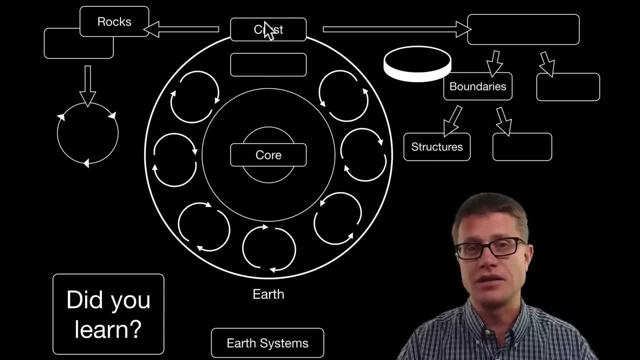 You are going to have to do some research. You are going to have to do some research, not I would say. we have a center core, We have a mantle and a crust. The crust is made up of rocks, which, in turn, are made up of minerals, which is reshaped using the rock cycle. These 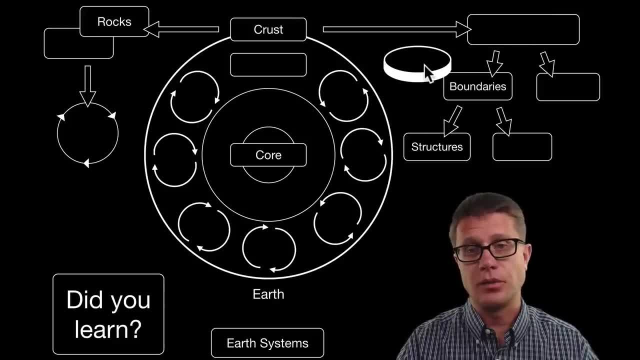 plates move on the surface. We call that plate tectonics. An example would be the ring of fire. Where we have boundaries, we can build up structures like volcanoes, mid-oceanic ridges, But we can also have natural hazards. And then remember, not along boundaries, but